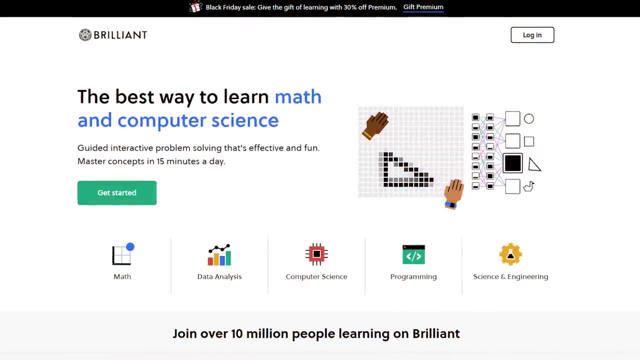 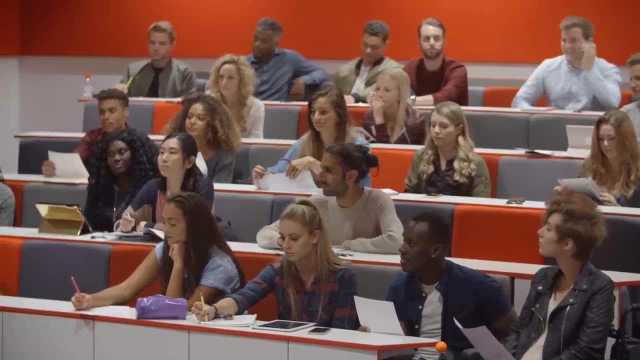 or a website called Khan Academy. I mean, you can even learn most of what you need on brilliantorg- sadly not sponsored- or you just go to college and take the mandatory maths classes for any engineering major. I'll tell you about my absolute favorite resource for learning: the. 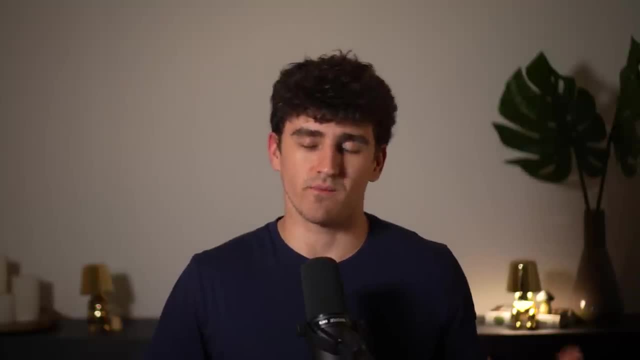 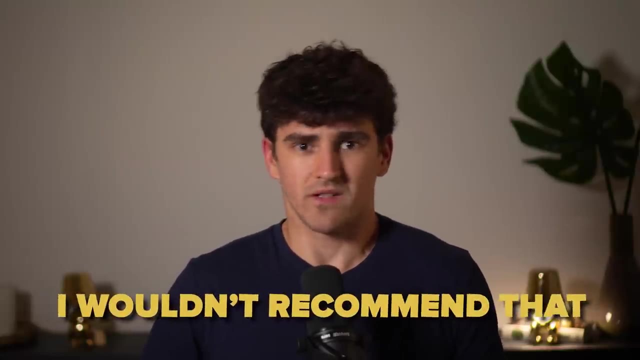 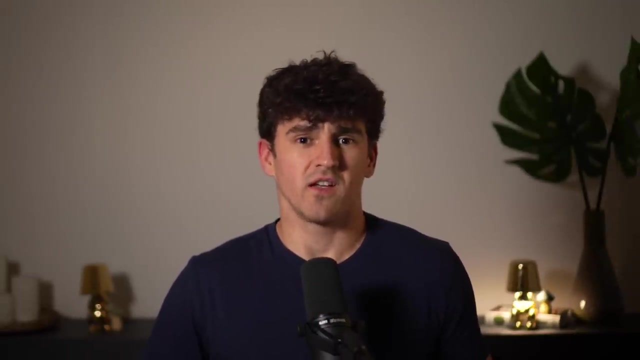 fundamental maths for neural networks after we cover the next important step. This already shows you that you don't need to hustle through all the maths courses there are in the beginning. In fact, I wouldn't even recommend that, because it can be very frustrating and just not fun. Whenever you don't understand some maths later on, you can always. 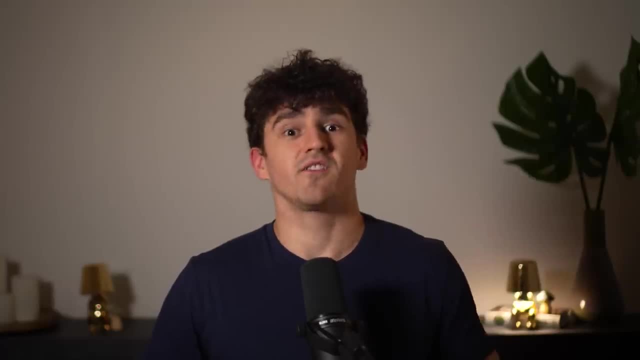 revisit it by just googling. Learn the basics and then continue on to the next fun step, learning about the ML Developer Stack. So now you know the basics of Python and, if you haven't already, can learn some basic tools like Jupyter, Notebooks and libraries like 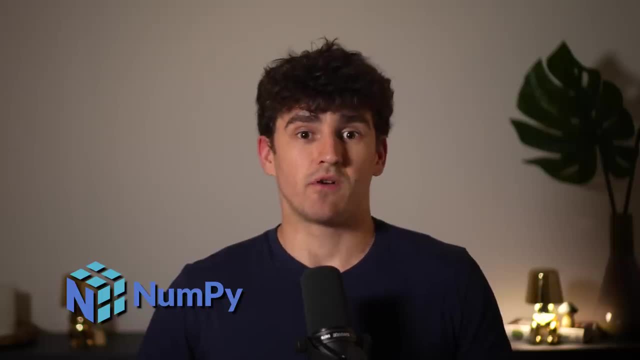 Pandas, NumPy and Matplotlib. NumPy is a library for doing maths with matrices or arrays. It's a great starting point because you can now implement the maths that you just learned about and see how simple it is to compute a dot product between two matrices. Matplotlib is a tool for visualizing. 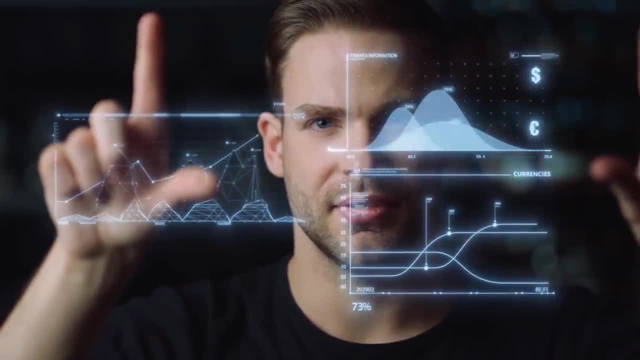 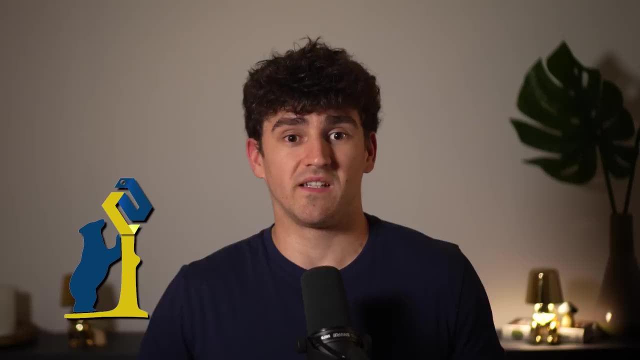 data and graphs and just seeing what maths you are doing- And, in my opinion at least, visualizing stuff is fun and just very useful. Finally, Pandas is a great tool for dealing with data that is in tabular format. Pandas is a great tool for dealing with data that is in tabular format. A lot of 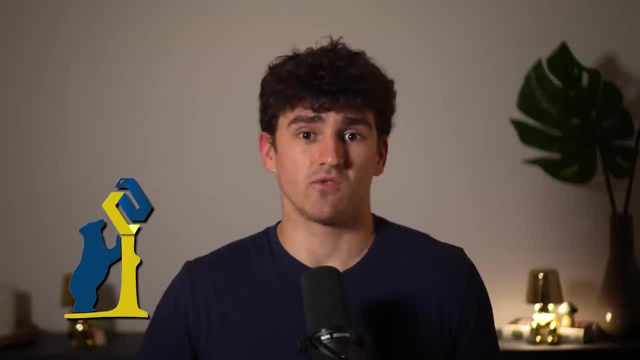 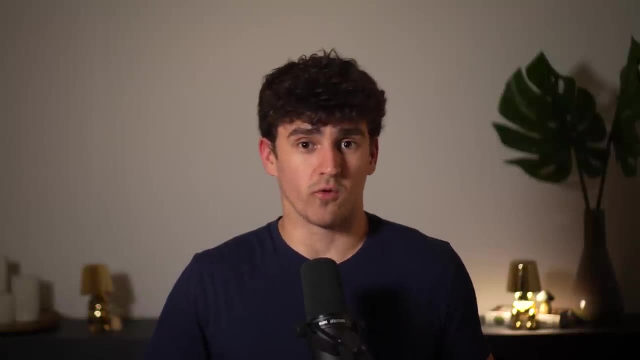 machine learning problems deal with tabular data and Pandas lets you again very easily manipulate those and visualize the tables. All those libraries also work very well with Jupyter Notebooks and are an essential part of learning machine learning, As you will see, by getting to know those frameworks. 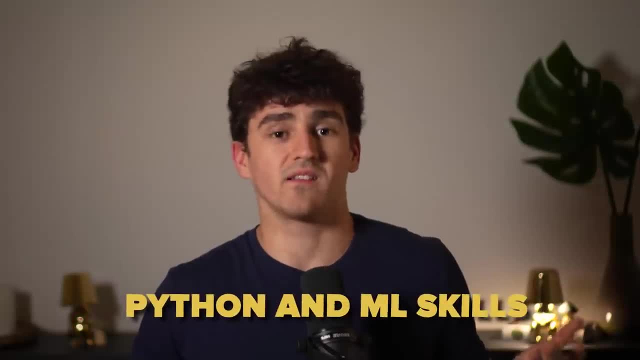 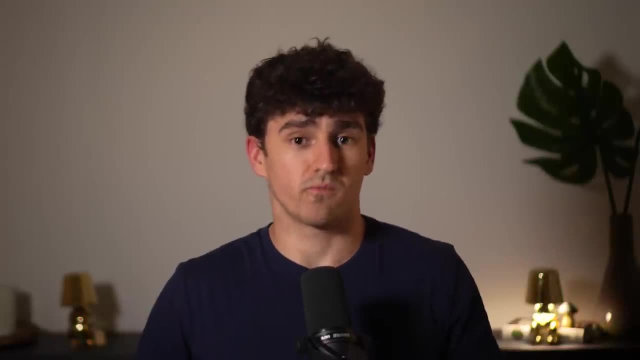 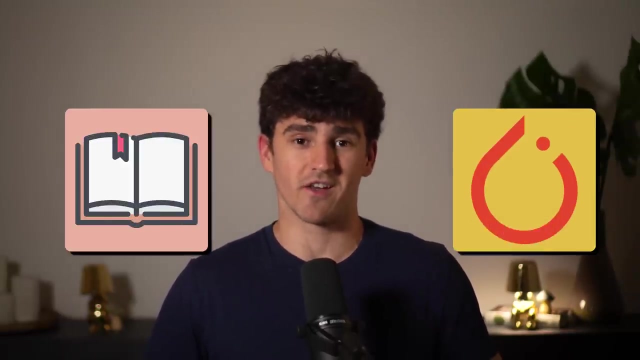 you will automatically improve your overall practical Python and ML skills. But again, only focus on the basics by following a few tutorials. Later, when working on projects, you will really get to know the libraries. So now let's get started. Let's get back to some theory and finally actually learn about machine learning and deep learning. 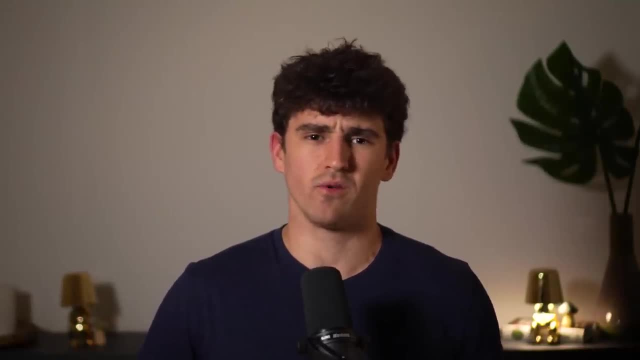 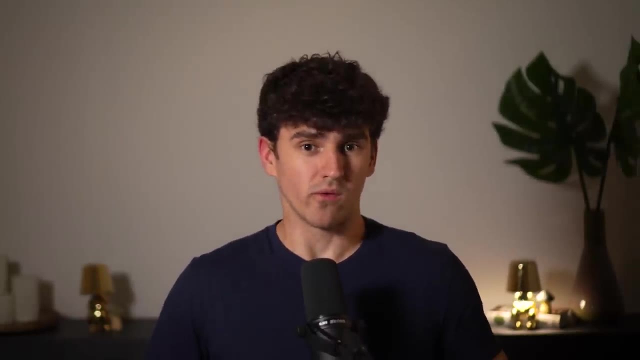 Okay, up until now, everything should honestly not take too long- perhaps a few weeks, depending on how much time you put in and at what level you already are. But the ML courses I will now recommend do take some time. The best and probably most famous machine learning course: 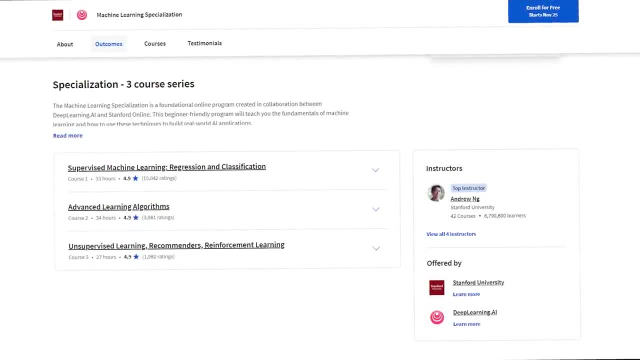 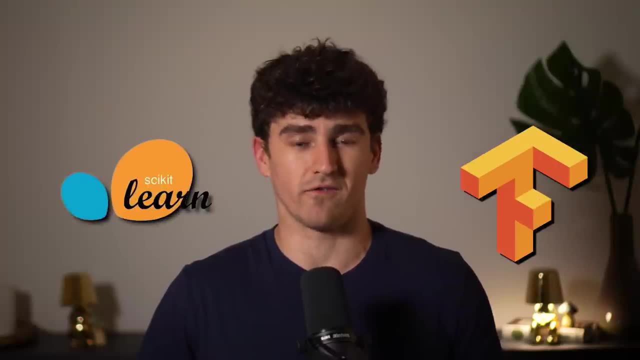 or collection of courses, is the Machine Learning Specialization by Andrew Ng. The cool thing is that you here already get to know some machine learning frameworks like scikit-learn and tensorflow. Well, I do have to admit I personally prefer and would recommend PyTorch. 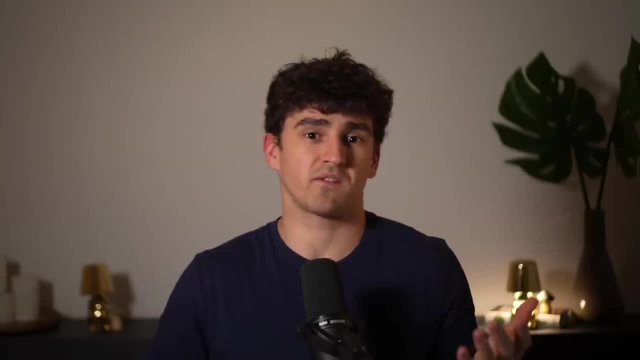 but learning one framework pretty much lets you already quickly adapt to the other one. This course is absolute gold and it's free. Although this is the beginner course, it is still very important. They here teach a lot of classical ML concepts, and those are the. 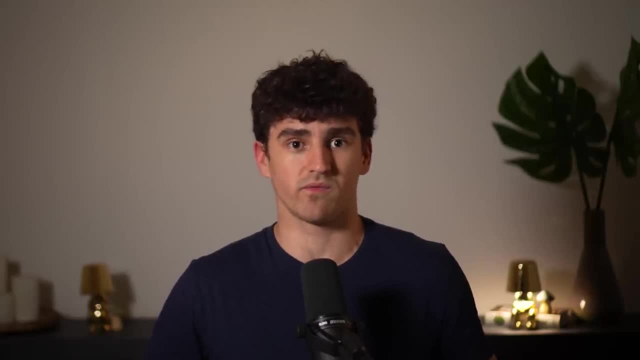 things you need to be able to answer quite easily in ML interviews. Now remember when I teased my favorite resource for learning maths in neural networks. Well, after learning about those in Andrew's course, I would watch Andrej Karpathy's Neural Networks series. 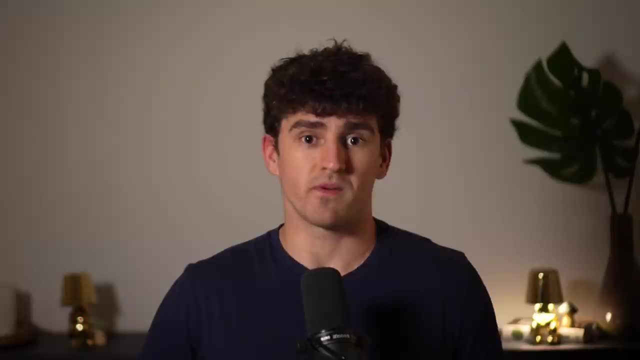 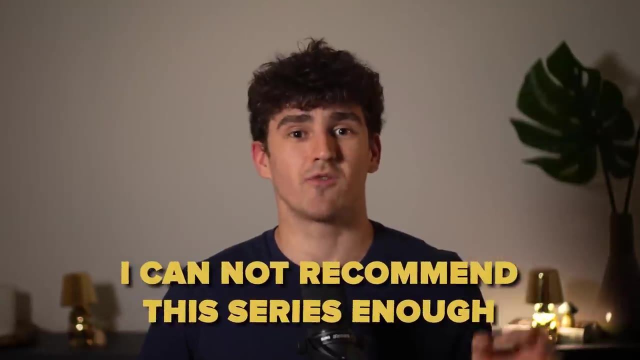 He here implements a simple NLP model from the ground up and goes all the way up to a transformer model. He also goes through all the maths of backpropagation and so on. I cannot recommend this series enough, Since in Andrew Ng's and Andrej Karpathy's courses you already get some. 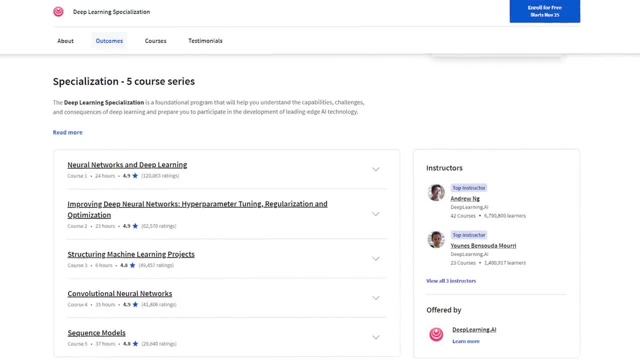 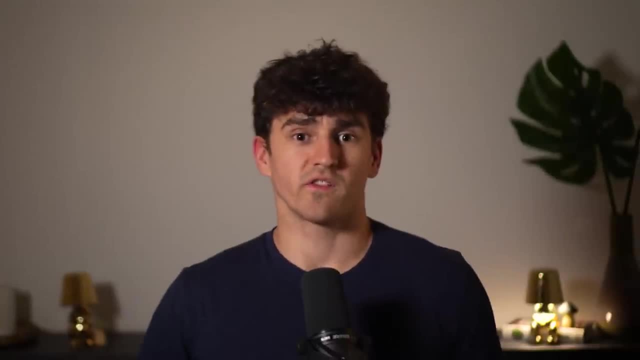 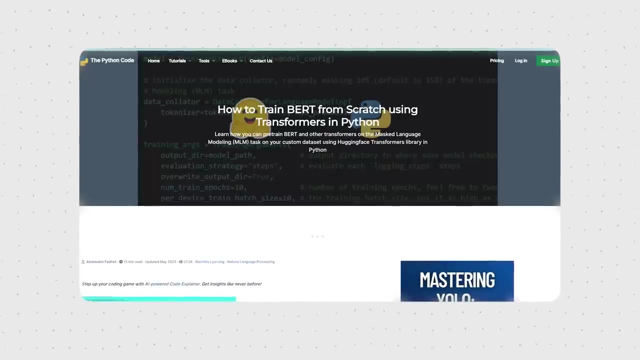 practical experience with the taught ML concepts. I would then continue on to the next, more advanced learning specialization. This course focuses more on implementing and training neural nets, and the absolutely amazing thing here is that they also include Hugging Face, which is a library that you pretty much 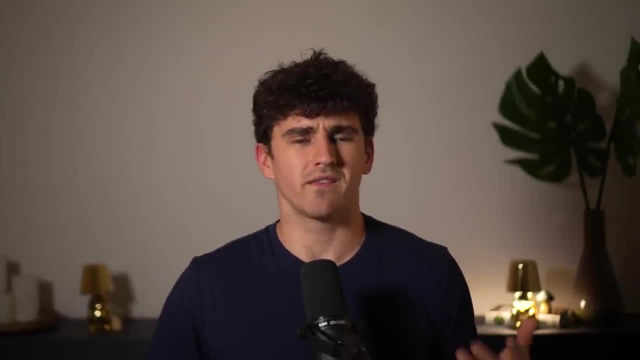 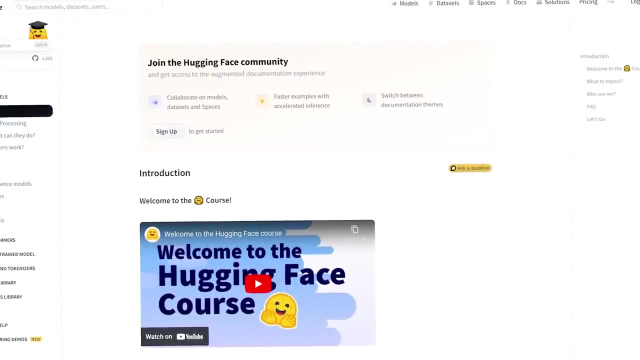 cannot avoid. It's really amazing, And if you feel like this course doesn't teach you enough about Hugging Face, you can also just go through the Hugging Face NLP course directly. There you also learn even more advanced concepts in NLP. Well, if you are interested in NLP. 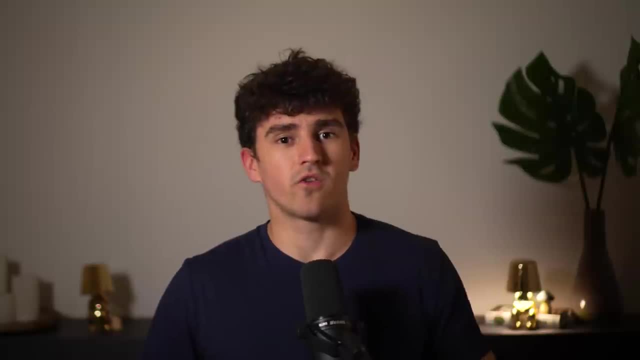 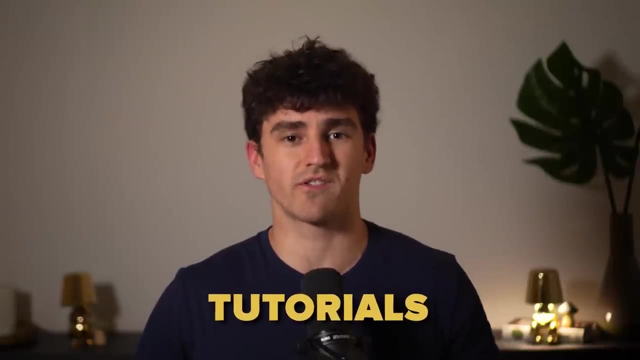 that is So. yeah, those are the two or perhaps even three courses I would recommend you to take and recommend. By now, you have learned a lot and worked on several smaller projects, or rather tutorials. Now it's time to actually get your hands dirty and work on real projects. I honestly 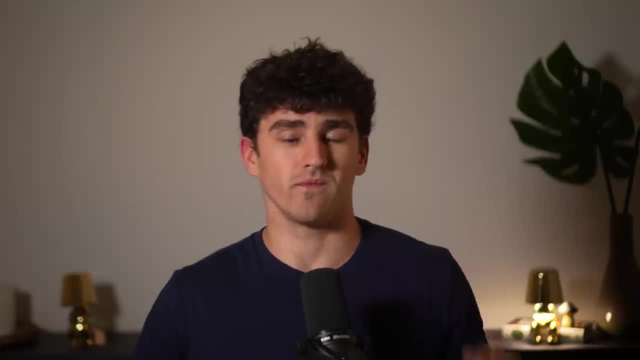 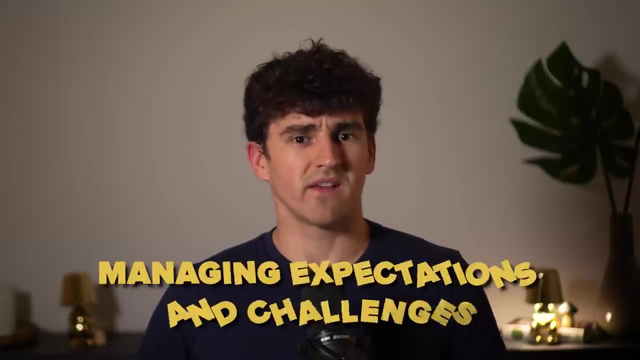 think you here learn the most, and there are two things I would work on. First, I would go to Kaggle and just work on challenges. There are many available for any level. Try not to underestimate the complexity and start with simpler challenges so you don't get frustrated.